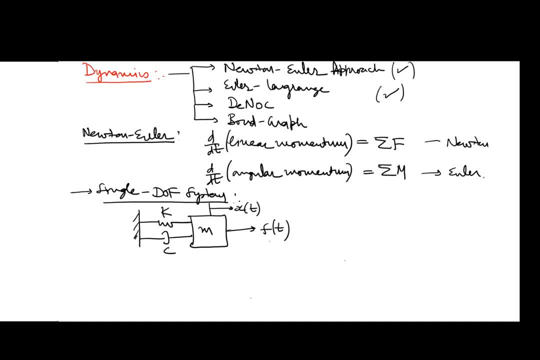 element. the function of this element is to oppose the displacement occur in the mass. So that's a function of displacement. and the function of the damper is to oppose the velocity. So any single degree of freedom can represent many examples in the nature. So, like we can say, if it could be a. 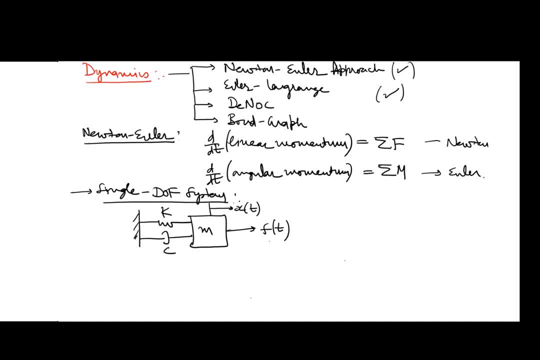 suspension system. it could be a car model, it could be a plane model, it could be a train model, it could be a model of a building. So, like you are having a building having multiple floors, So this building can be represented by simple spring mass damper system. It could be like Burj Khalifa. 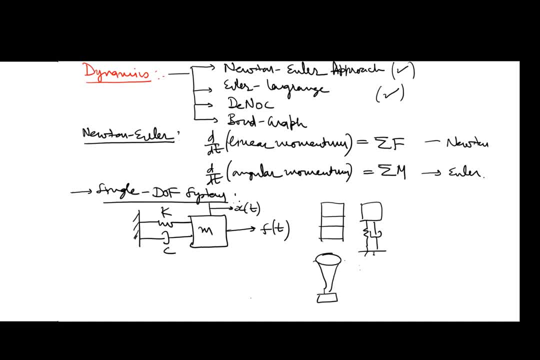 so where there is a huge tower, So this tower can be represented by, again, single degree of freedom system. So single degree of freedom systems are extremely important from the point of view of its simplicity and with which we can relate many examples in day-to-day life. To develop its equation of motion, typically write the equations like this way: 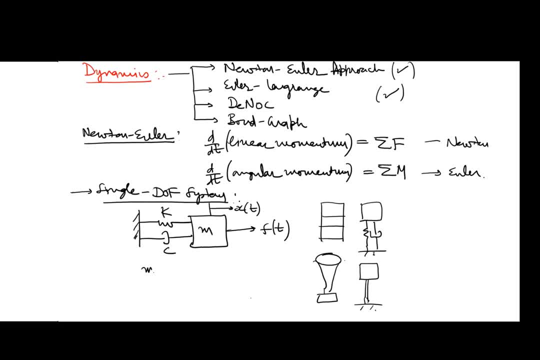 mx, double dot plus cx, dot plus kx, equal to f of t. But that is not the correct way to write it. We have to follow the procedure systematically. Eventually we will come to this equation only, but we should know clearly that what are the sequence of steps which are involved to 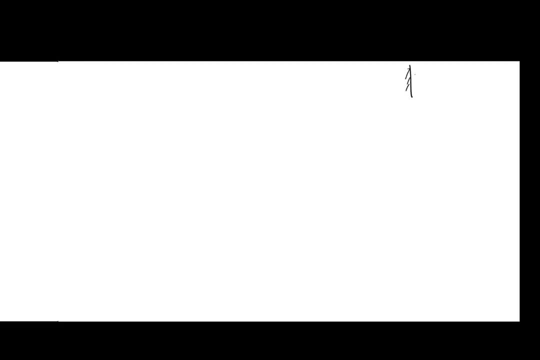 reach at this equation. Let's draw this figure again. So we are having this x of t and then you are having f of t. This is the external force applied to the system. So only thing we need to understand is what is the meaning of this x of t? The x of t is a displacement, but it is given. 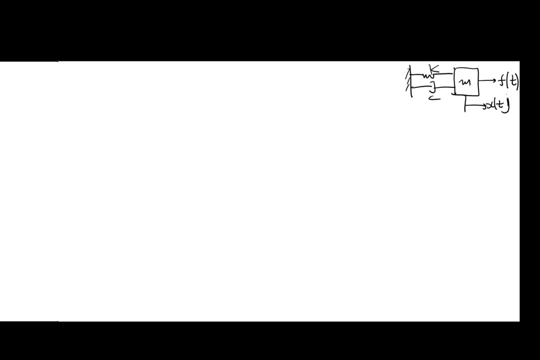 a specific name. It's called as the displacement from the mean position or the displacement from the static equilibrium position. The first step in this is we need to develop its free body diagram, where we isolate the system and will represent all the forces acting on this like there is a force f. 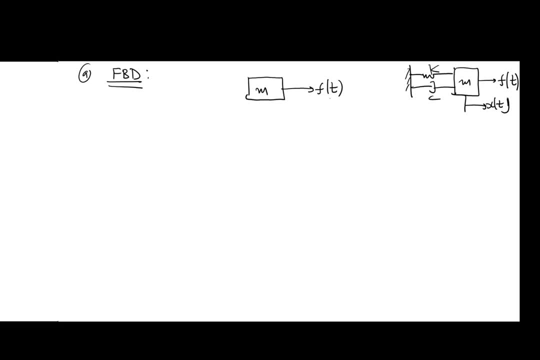 there is no mg force, So as the body moves to the right, the spring will try to oppose the body in the left hand side. This is called as the force due to the spring and because the spring tries to oppose the motion or displacement of the body. that's why it's kx, Whereas the function of the 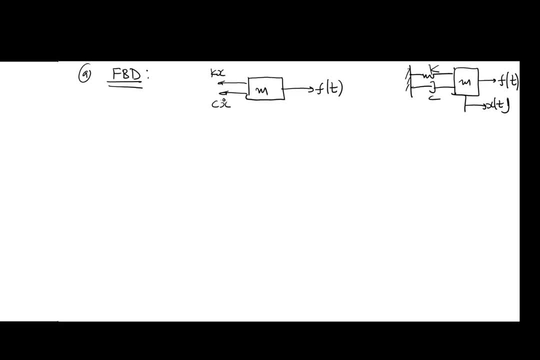 damper is to oppose the velocity that is cx dot. So secondly, we need to apply Newton's second law, the rate of change of linear momentum. So in this case we have m and the velocity of this body is x dot is equal to summation of all the forces. 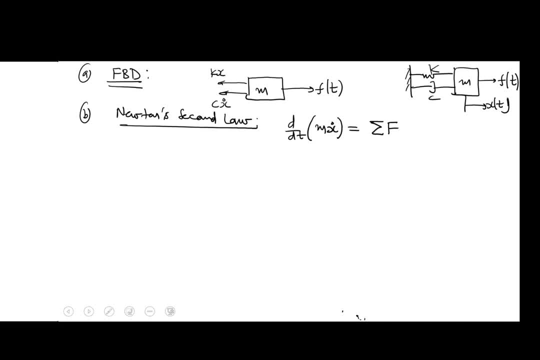 acting on the system. These are external forces. So now we have to have this assumption. Otherwise we have the derivative as m dot, x dot and m x double dot. but we are assuming over here because this is a normal derivative in such situations where we cannot ignore the rate. 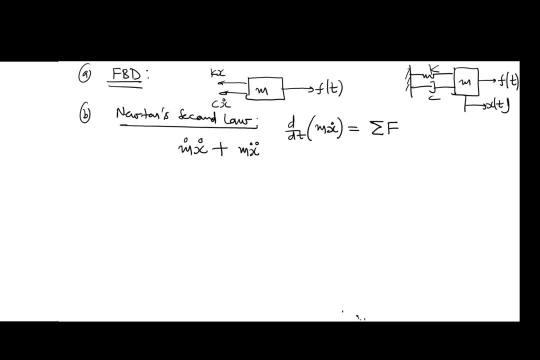 of change of mass also. So this is under the assumption that in 95% of the cases the mass of the body under concentration will remain constant. So in that case, this term the rate of change of mass will go to zero. but otherwise, if it is not being mentioned, like in the case, 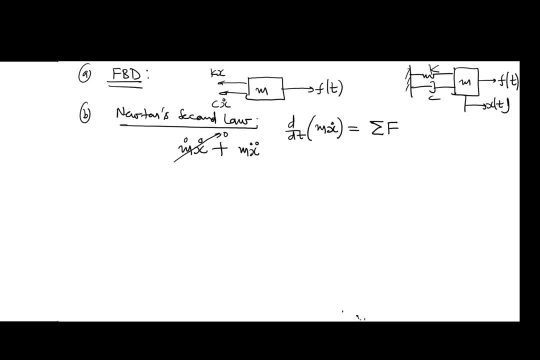 of a missile which is going to hit the aircraft, the mass of the missile is changing drastically. So in that particular example you cannot take that as the assumption. So in most of the cases the mass of the system is considered constant. So that's why we have this. 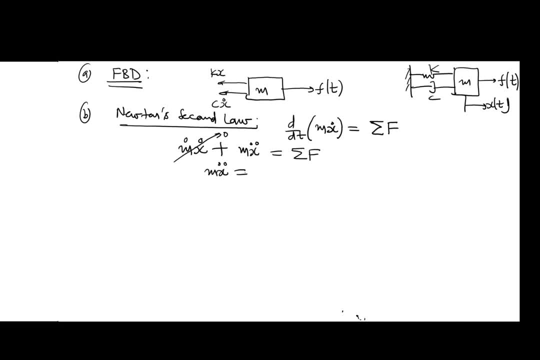 So then you have m, x, double dot. So if you now see the free world diagram, all the forces towards the right hand side will take it as positive. So F of t, that is external force, minus K, X, the spring force, minus c, x dot the damper. so then the step C, we'll say collecting. 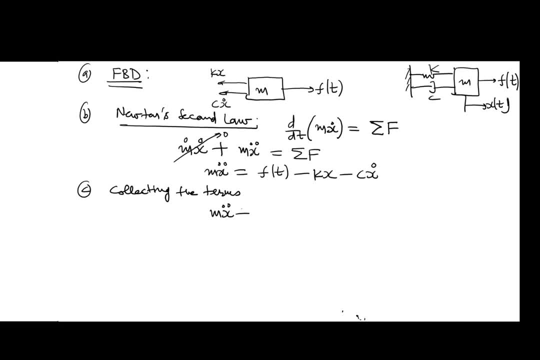 the terms. So we have m, x, double dot H, e. So that's what we have. Once we get the m, we take it as D 볼 and gives the shear. but now that we have idea, Now that we have, 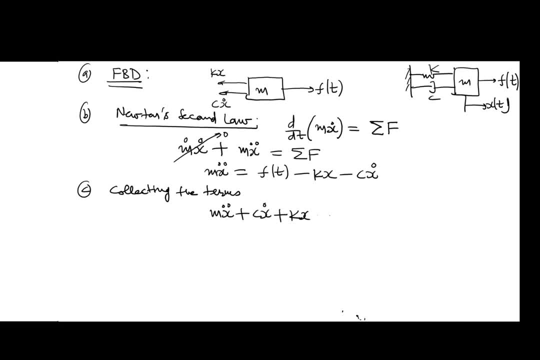 plus CX, dot plus KX, equal to F of. So this is what we have as the standard equation. Now let's reorient the body and let's try to see what will happen when the body is something like this in the vertical position, where everything will remain the same. Now, if you draw its, 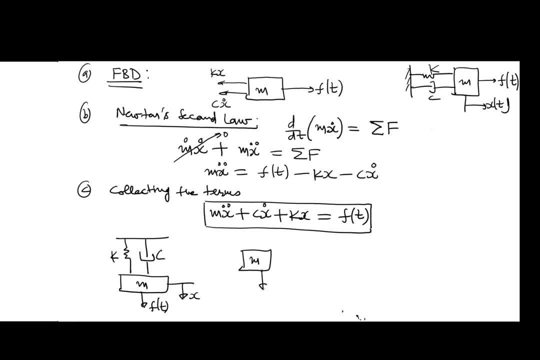 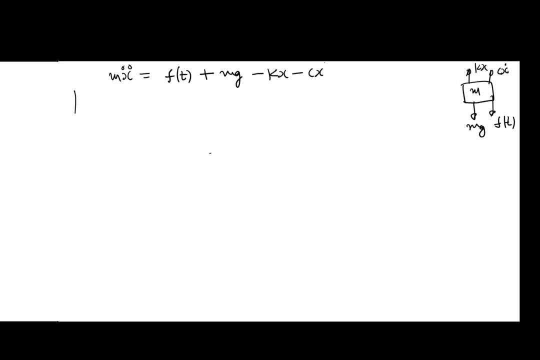 free body diagram. so same thing will come. So you are having a Ft force, KX force, CX dot force. Any other force will come, Gravity force will come- Mg, right. So now, if we again write the equation of motion, in that case we have F of t plus Mg, minus KX, minus CX dot. 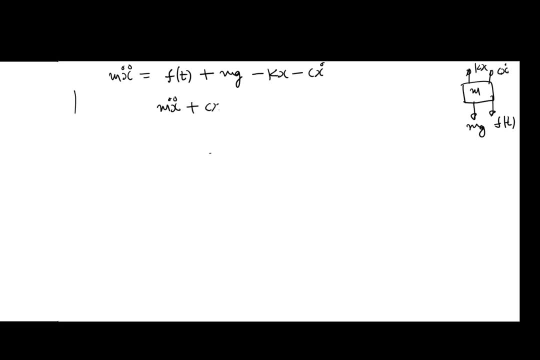 So in that case our equation becomes Mx double dot plus CX, dot plus KX, equal to F of t plus Mg. right, This is what we will get as the equation. This equation is wrong. The wrong part lies that there is no Mg term will come, So the reason lies over here, because the displacement 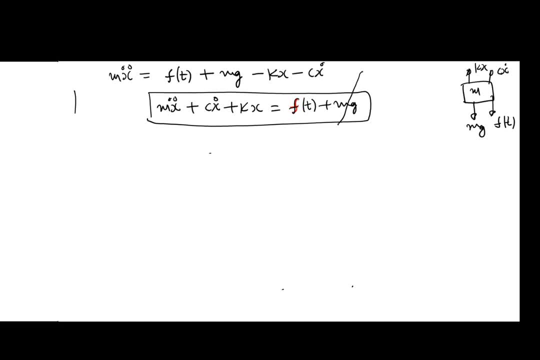 mentioned over there is the displacement from the static equilibrium configuration. So where this Mg goes, let's try to see- You have a mass suspended on a spring. spring will vibrate and the system will come to rest after some time and thus this delta static will be there. 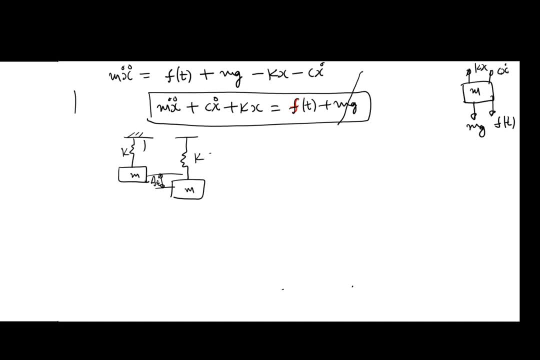 the deformation in the spring. so if we draw the free body diagram now, so you can see mg equal to k delta static, so that is the static deflection. at static equilibrium we have mg equal to k delta static. that will come. so now if you further draw the spring by xt amount, so now the spring will 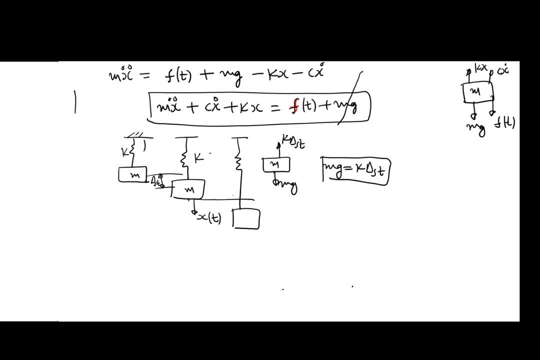 open by this much amount xt more. so now, if you draw the free body diagram, you will see, because of this force due to which this xt happens, the spring will actually elongate by x plus delta static. total delta static is already there because of mass m, and now x displacement is there because 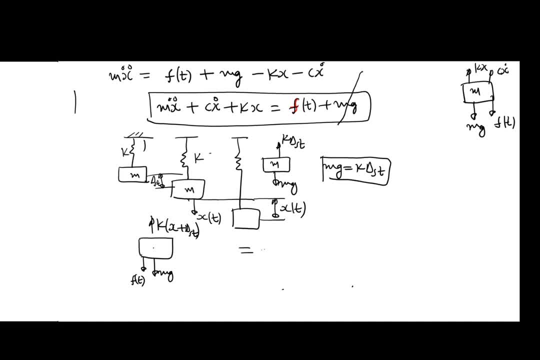 of this force. so now you will see this. forces are opposite. so ft plus mt, g minus kx, minus k delta static. but from the static equilibrium we can always cancel k delta static with mg. this will happen every time, so whenever there is a spring attached, so the mg 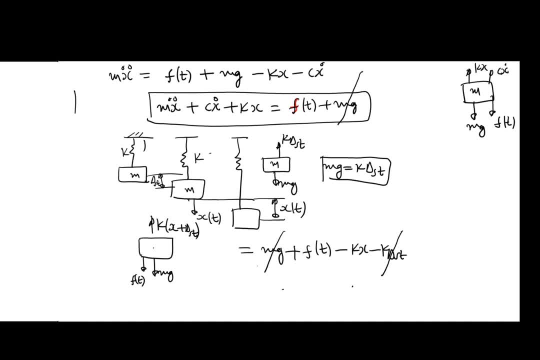 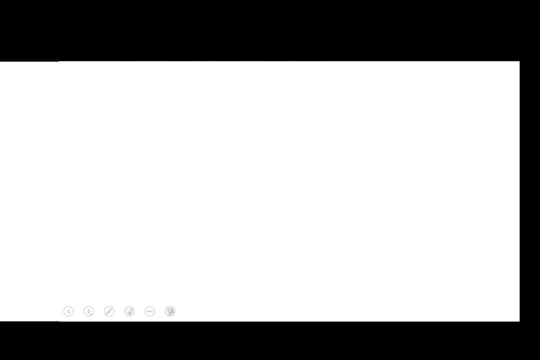 force will be compensated automatically. so we need not to take into account the mg force. so the equation of motion will remain the same: mx, double dot plus cx, dot plus kx, equal to f of t. so let's see the general case. the general case is the one where the 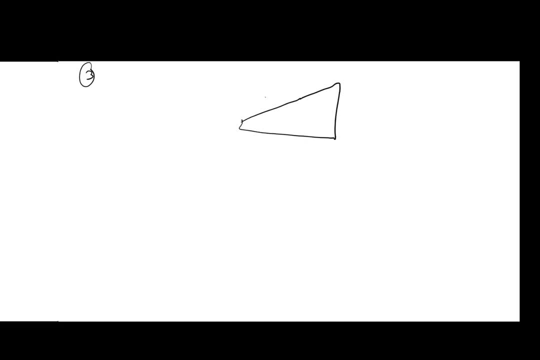 spring mass damper system is on inclined wedge. so now you have this system having mass m on wedge where the angle is phi. so you have mg force, so this angle is phi. so we know this component is mg cos phi, this component is mg sine phi and there is a spring and 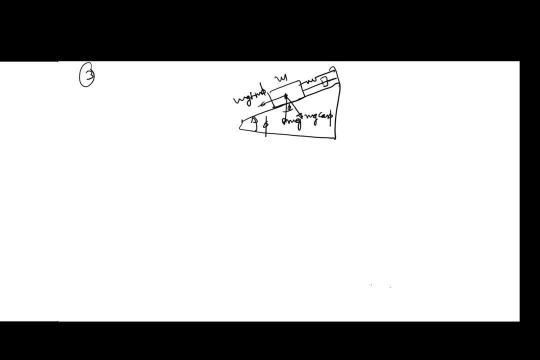 there is a velocity at which the senator will get balanced with the weight of the spring mass. so that is it regular equation with the same thing, k and c. at the static equilibrium, mg sine alpha will be balanced by k delta static. so what will happen now? we have three cases in all those. 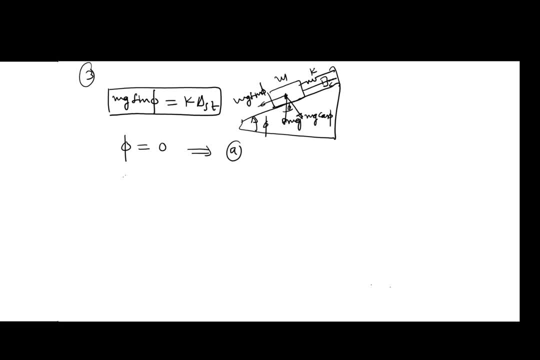 cases, the equation of motion will remain the same. if phi equal to 0, that results the first case. when the system is horizontal. when phi is equal to 90, that results to the second case, when the system was vertical and when phi is arbitrary and when phi is arbitrary. 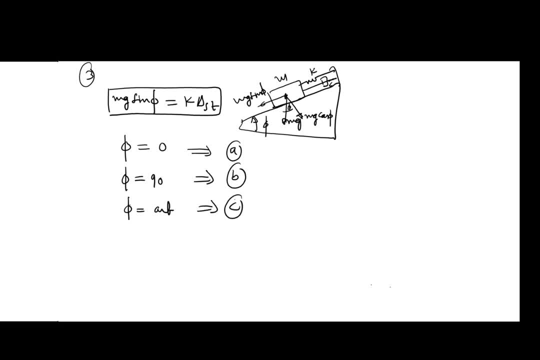 this results to the third case, when the system is inclined. so this phi is generalizing basically 0, 90 degree or arbitrary angle, but we have to take care. so whenever there is a spring, either vertical or inclined in the system, that spring will take care of the static loading. so the mg 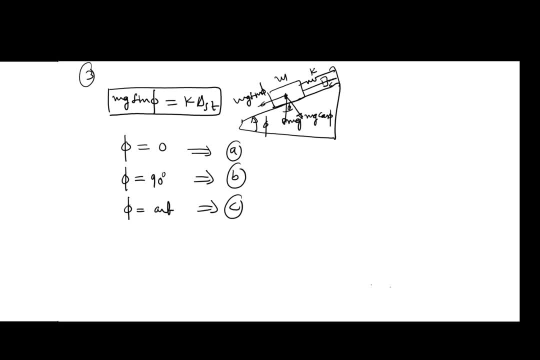 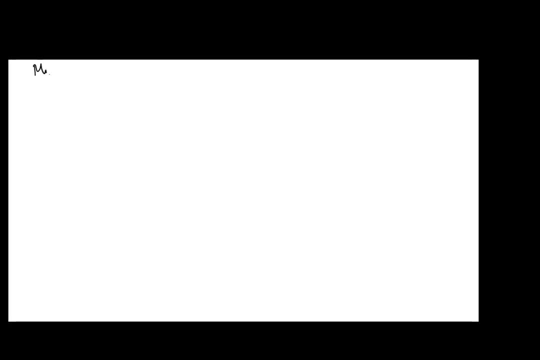 force will never come into count. that is the significance of saying that we are taking the displacement after achieving the static equilibrium conflict. so we'll switch to multi-degree of freedom system. for the timing, let's take two degree of freedom systems. from this we can generalize and we can go to the multi-degree of freedom. so let's take the example. 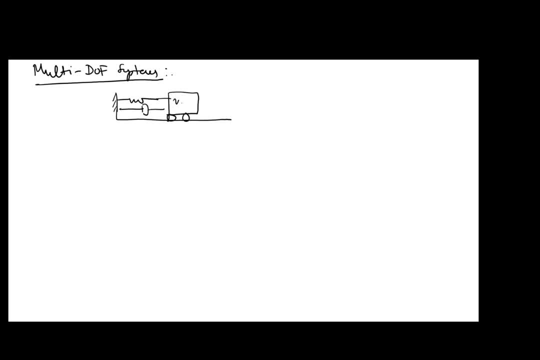 same spring mass damper system. so let's, we are having a body m1, there is a body m2, there are two bodies. this kind of system can represent something like tram in amsterdam, or there are trams in kolkata also. this displacement is x1. this displacement is x2. 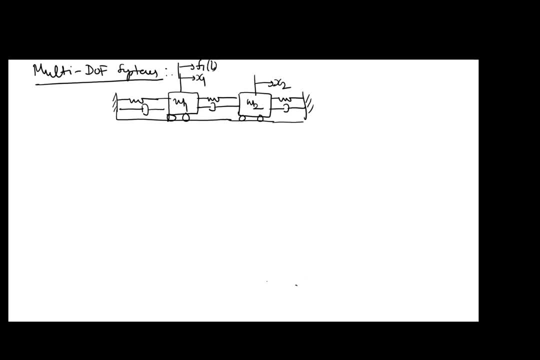 the force applied on the first body is f1t, the force applied on the second body is f2t, and let's say there are three springs involved: k1, k2 and k3. and then there are three dampers involved: c1, c2 and c3. so before going this type of a question we have to take first thing is the 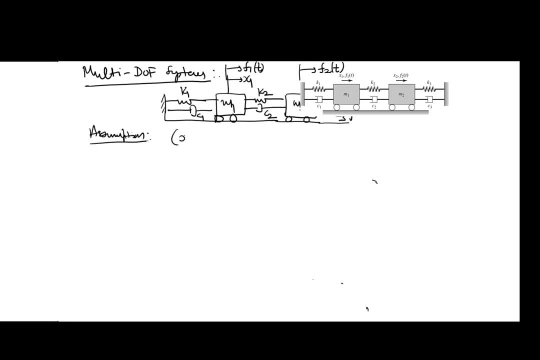 dimension, so we have to take into account which type of case we are considering. either x1 is greater than x2 or x1 is less than x2, so this will help us to draw the forces and their arrows, or their directions, in the correct manner. as i mentioned, the first step is we need to draw the 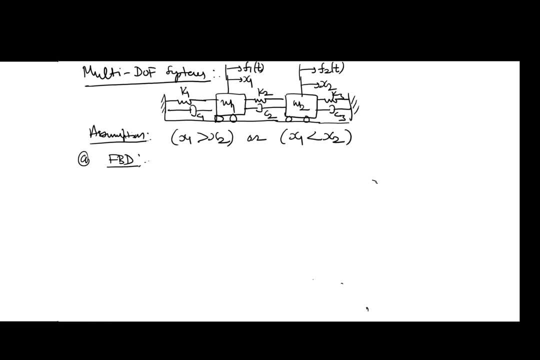 free body diagram. so in free body diagram for multi-degree of freedom systems, especially the system where there is a coupling existing between the two. so it's always better to draw the free body diagram simultaneously. so this is a body one m1 and there is a body two m2. let's see. 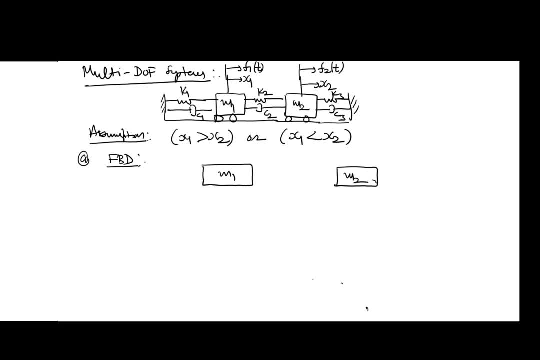 the first body, m1, so the first body we can say: when the body goes to the right, the spring k1 is under tension, so it will try to pull the body back towards the left. that's why that's the force kx. so whatever is the direction of x, the same is the direction of damper cx, dot. that is the one. and 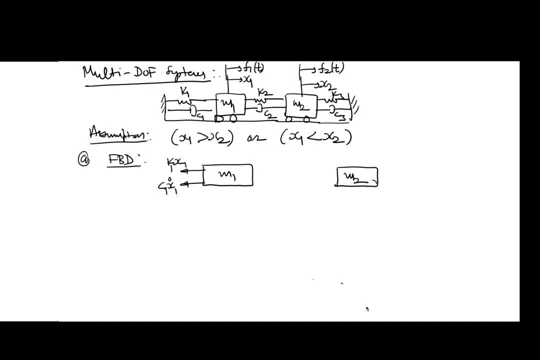 spring k3, or that is also a decoupled spring, only applied to body two. so when, under the influence of force two, this body m2 moves to the right, the spring, what is the state of spring k3? that spring is compressed. so when the spring is compressed and the tendency of the spring is to regain its, 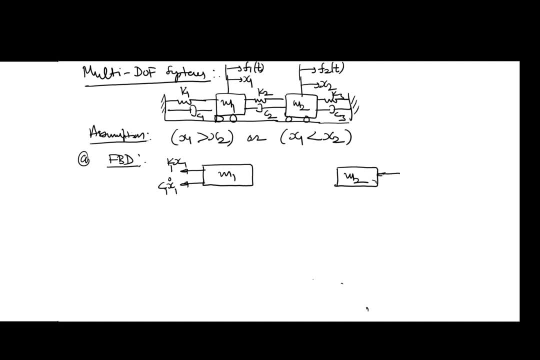 original position. this will push the body backwards in the left hand side and the force is k3 x2 and the force acting on this due to damper is c3 x2 and certainly there are two forces acting on the system. f1 is also there and f2 is also there. these are the forces due to external force. now comes the tricky. 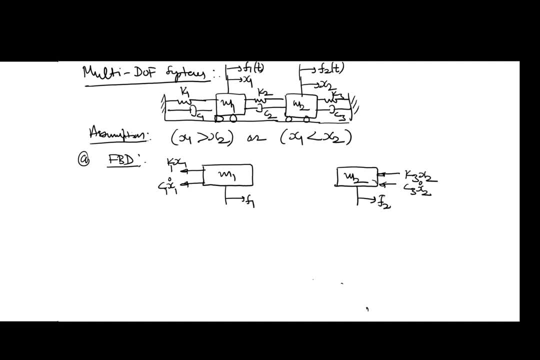 one, the spring k2. the spring k2 is a coupled spring because it's both the free ends are connected to two movable objects, whereas in the case of spring k1 one end is fixed, one end is attached to the body. same is true with spring k3, where one end is. 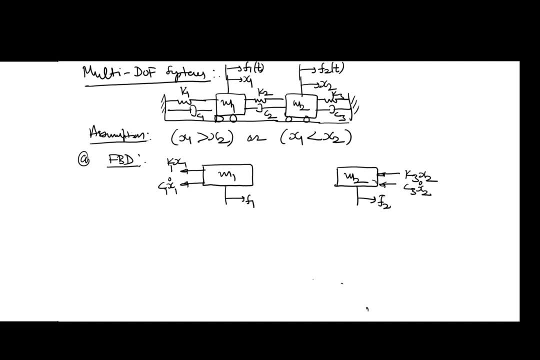 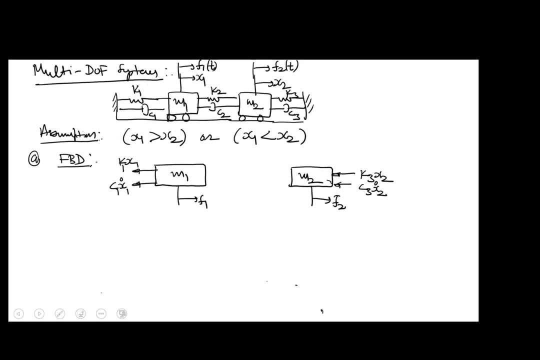 attached to the body m2, the other end is fixed, whereas in the case of spring k2, both the ends are attached to two movable bodies, m1 and m2. that's why, in order to detect its state, we have to make this assumption. so let's take this assumption first. x1 is more than x2, so now you can assume. 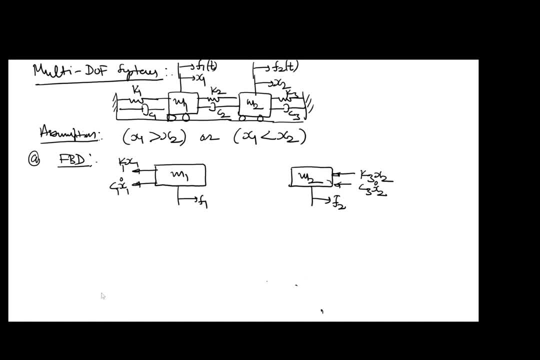 if x1 is more than x2, let's assume both you are having two bodies and both the bodies are moving towards the right. so what will happen after a period of time? because x1 is more than x2, so the both the bodies, while moving towards the right, will come closer to each. 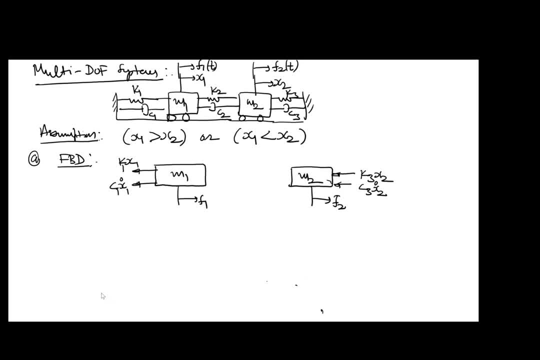 other, the distance between the bodies will keep on reducing, so, which means the spring k2 is under compression. so when the spring k2 is under compression it will apply a outward force, k2, as x1 is more than x2, so x1 minus x2. so that's why these two arrows pointing outwards. 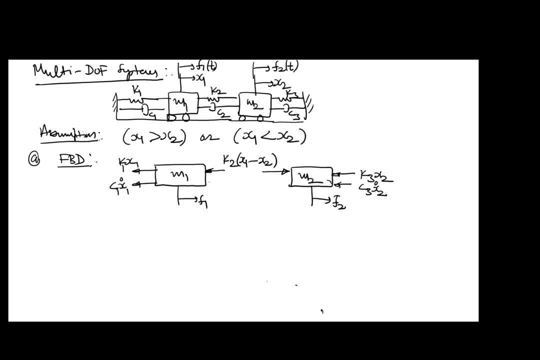 their direction is very important. same thing is true for the damper. whatever is the direction of spring, the same is the direction of c2, x1, dot minus x2, if we have taken this as the assumption. so i'll draw the free body diagram again in red color. so the same thing will happen: m1, m2, nothing will be different for the spring: k1. 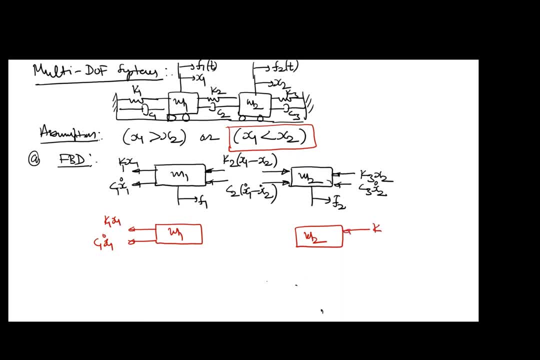 and nothing will be different for the spring k3. all those forces will remain same. the only difference lies in the middle spring, where now there is assumption different now because x2 is greater than x1. so when both the bodies are going towards the right and x2 is having more displacement, you can see the distance. 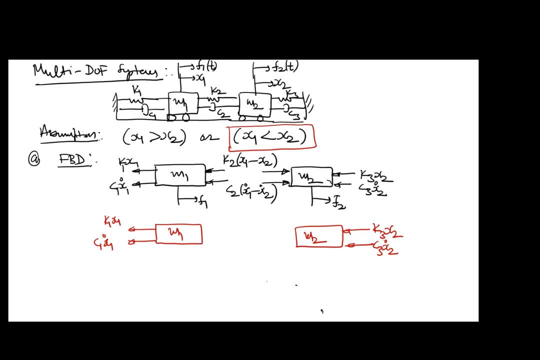 between the bodies will keep on increasing. so as the distance between the bodies will keep on increasing, the spring k2 will come under tension. so once it will come under tension it will pull both the bodies inwards and the amount of force is k2 into x2 minus x1. 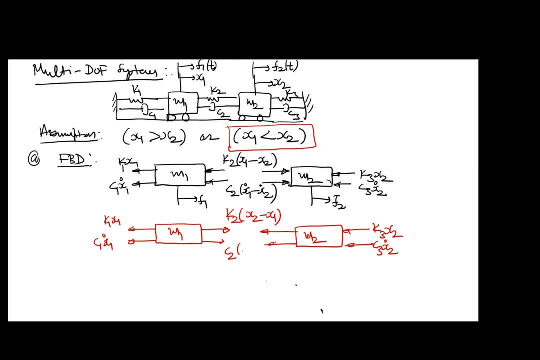 and same thing with the damper c2 into x2 dot minus x1 dot. now you can see: eventually, either this force and this force. there is a minus difference and there is a change in arrow sign. so eventually, whatever assumption you will take into account, it will end up with the same force. 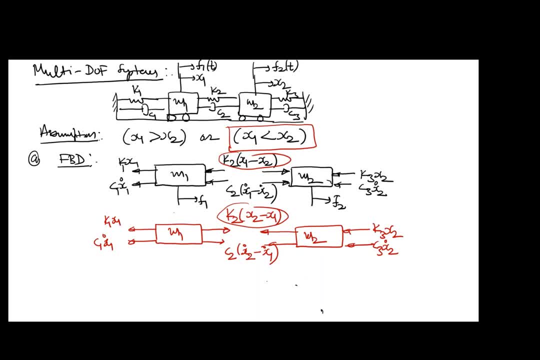 so because the equation of motion is a property of the system and this property does not depend on the force. This publisher does not depend upon any initial condition or any assumption. so, whether you take x1 more than x2 or x1 less than x2, only the arrows will change and the values will change, but eventually the force applied. 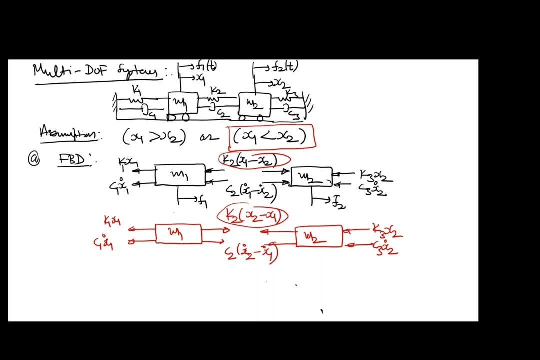 by the spring and the equation of motion in both the cases will remain the same. so let's consider the first case back and try to derive the equation of motion of the first case. well, go back with the black pen. whew, the assumption plays out very well. now the question�. 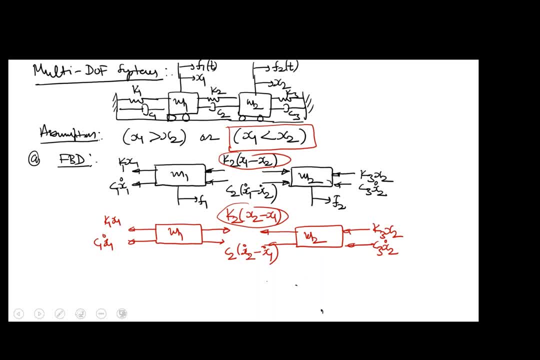 is whether x1 less than and opposite ratio is a problem, or because the less important thing is that always, in both cases, the française will not have the same same force. we are going to have a different force and therefore that will do not solve anything if x2 less than x2 does not depend upon the initial condition or any assumption. so, whether you 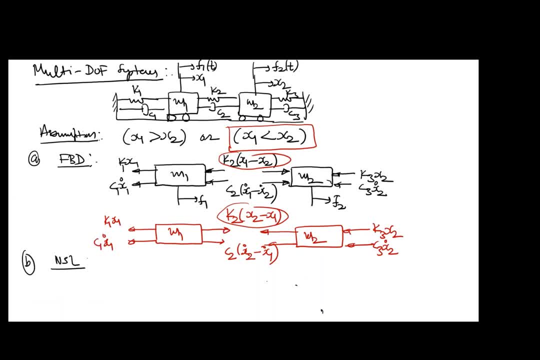 step b, where we have to apply Newton's second law. Newton's second law says d by dt of m1 x1. dot rate of change of linear momentum of the first body should be equal to the force f1 and all the arrows towards the left. so all are negative. so minus k2, x1, minus x2, minus c2. 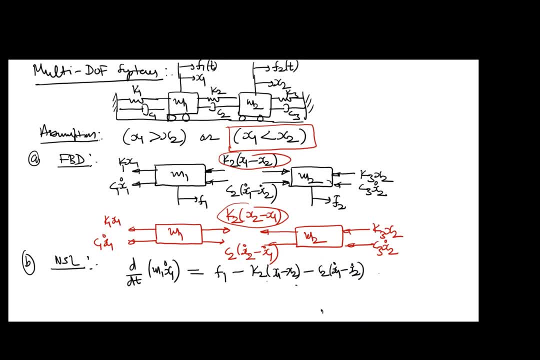 x1 dot minus x2 dot minus k1 x1 minus c1 x1 dot. so, on collecting the terms, we have m1, x1, double dot. so first we will have c term with x1, so you can see there is a term c1 x1 dot minus. 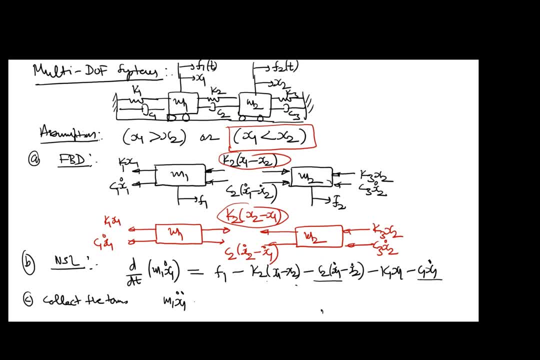 and c2 x1 dot minus. both will come plus and c1 plus c2. we can combine minus c2 x2 dot plus. so we have m1 x1 dot minus c1 x1 dot. so, on collecting the terms, we have m1- x1 double dot. 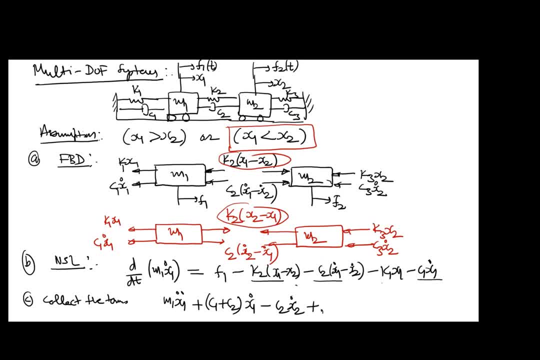 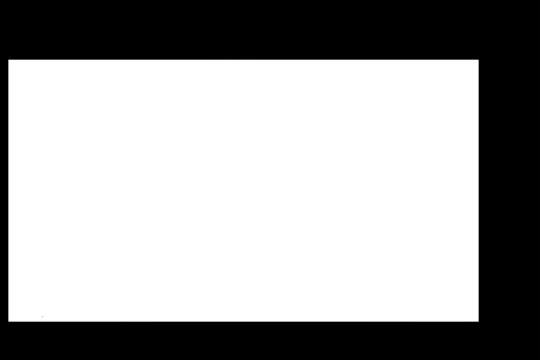 so k1 plus k2 times x1 minus k2, x2 equal to f1. so this is the equation of motion of the first body. so we will go to the next, so the free body diagram of the second. from there we can find out that d by dt of rate of change of linear momentum of the second body equal to minus k3, x2 minus. 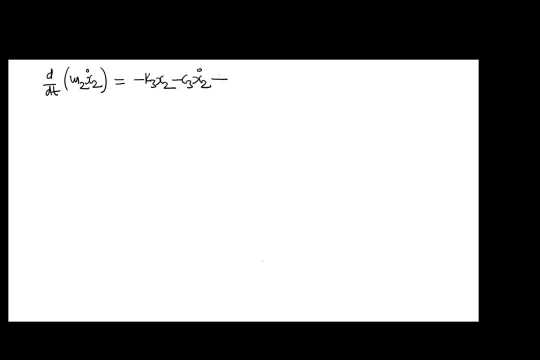 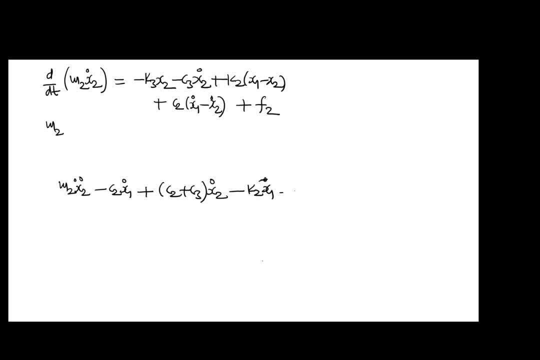 dot, sorry, not x1 dot, k2, x1 plus k2 plus k3, x2 equal to f2. so this is the equation of motion of the second board. now we can write them into the matrix form. so let me write the first equation first, which we have derived in the last slide, so that equation was m1, x1, double dot. then you have: 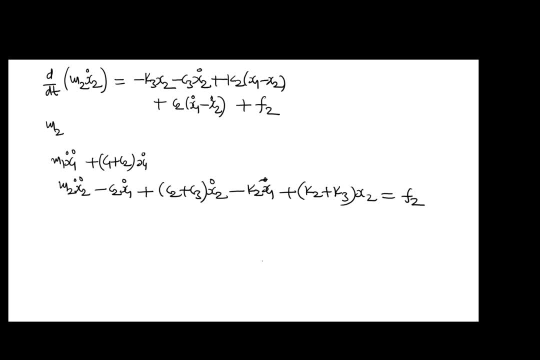 c1 plus c2 times x1 dot minus c2, x2 dot. then you have k1 plus k2 times x1 minus k2 x2, equal to f1. so that is the equation of motion, what we have derived in last slide for the first body. now we will see. for the scalar part we have the equation. 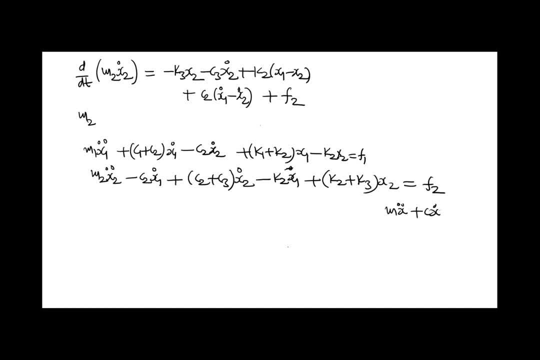 like mx double dot plus cx, dot plus kx, equal to f. so now for multi-degree of freedom. the structure of equation will remain the same. so instead of scalar m's we have now matrices: mx double dot plus cx, dot plus kx, equal to f vector. now let's try to see. now we have the vector of. 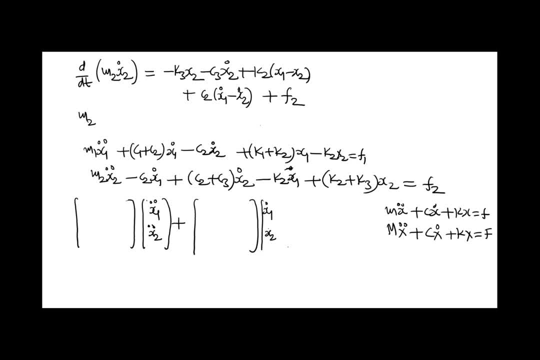